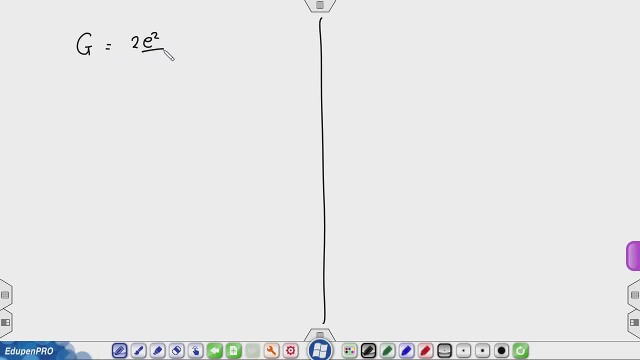 to speak, came in the quanta of E square over H times a number, an integer, And that means I can see that the resistance comes in the quanta of H over E square. This is the quantum, And where do we see it? very clearly It is seen in quantum Hall effect. So let me just 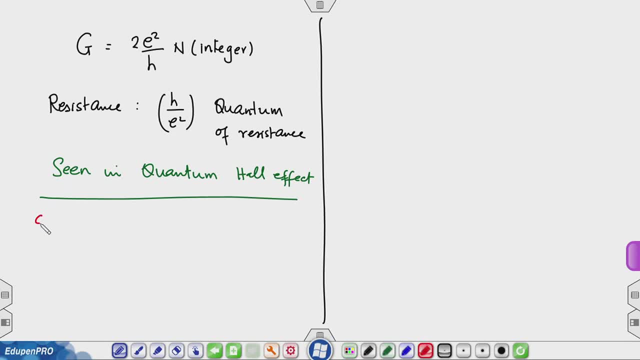 tell you what the experimental facts are about quantum Hall. First, one works in terms of a, 2, D electron gas. So I am making this diagram schematically and let a current- I pass through this- When that happens and you apply a magnetic field, 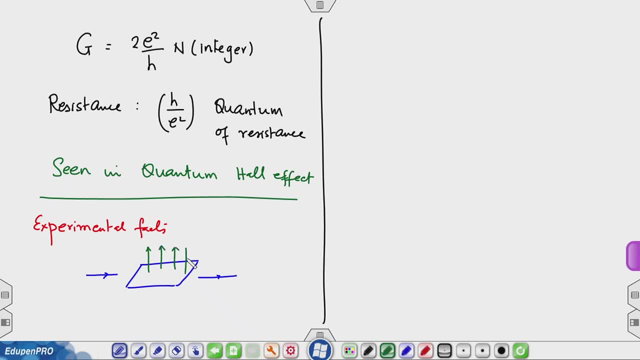 perpendicular to it. So this is a magnetic field. this is current I. you develop a Hall voltage across the sample. This is the experiment and what we had done earlier. this is the experiment. Now, let us recall, before we go any further, that resistance and resistivity for Hall effect. 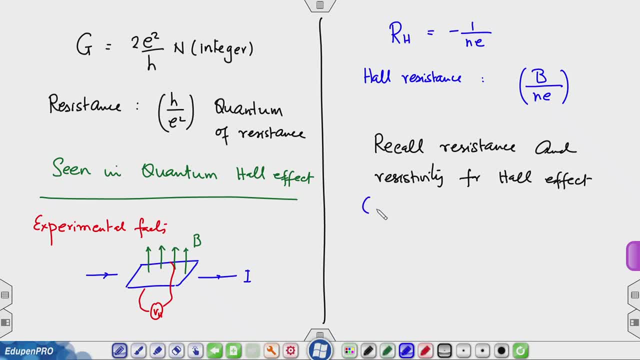 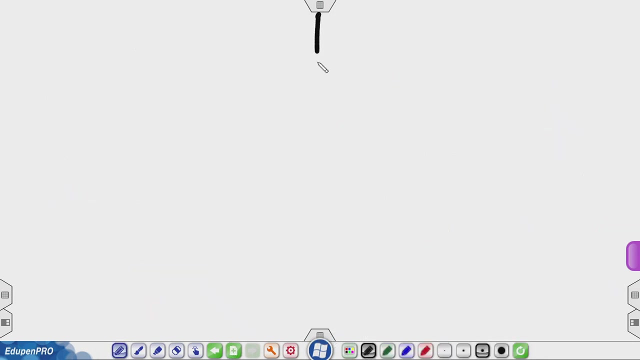 So, in effect, what I am talking about in proper language is Hall resistance and resistance. Hall resistivity are the same in 2 D. This was done in lecture 3.. So you do this experiment and usually what you see is that if you plot Hall resistance versus B, this, as I said, is: 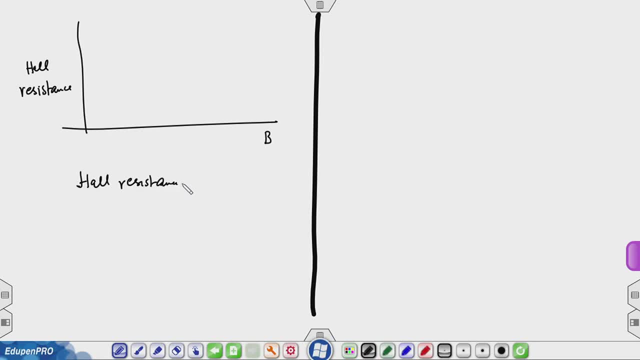 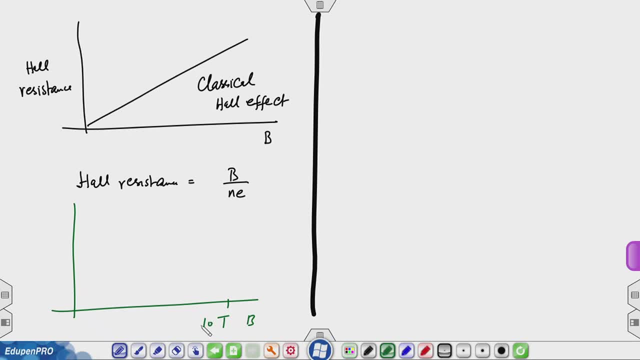 why this quantum Hall effect takes place and what is quantum about it? Quantum about it is that rho x, y, that is the Hall resistivity. 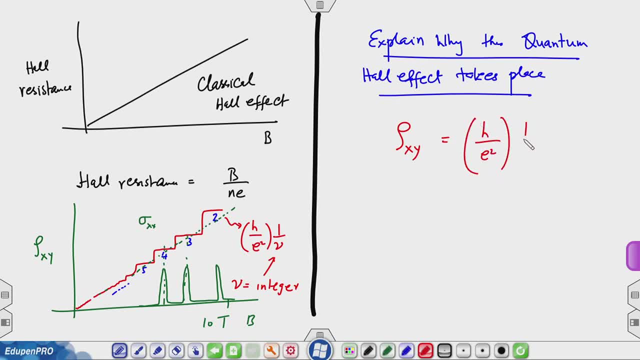 is h over e square and to a very high precision. this nu, where nu is an integer and in the play 2 rho, sigma x is the conductivity is 0.. So we will explore all this and try to understand why this happens. The explanation is quite simple, but the phenomena is so rich. 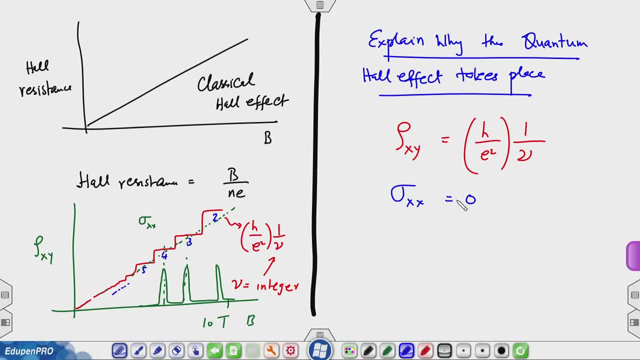 that it has given rise to many, many things. and further, one has also seen fractional quantum Hall effect, which we will not be going into in this course because that requires understanding interacting electrons. also, This can be explained through non-interacting picture. So first, what I am going to do is review what we know. 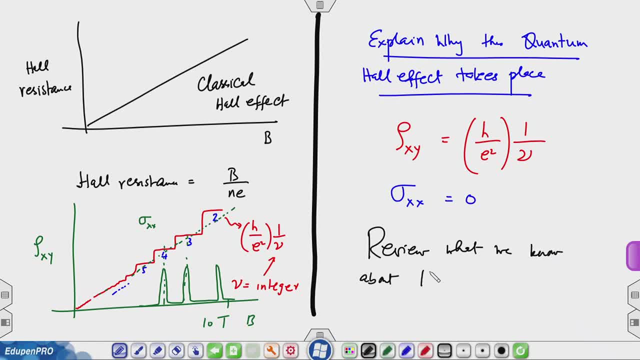 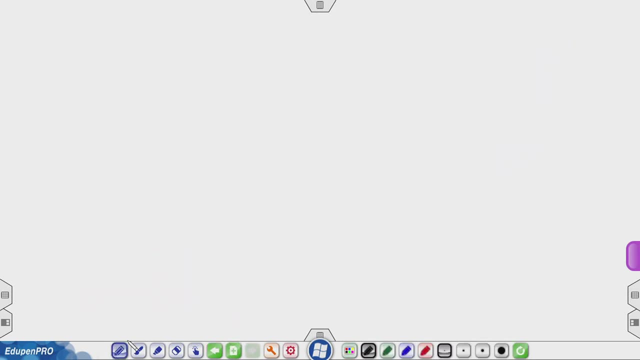 So we will learn about Hall effect classically and then we will connect it with quantum picture. You will have to keep going back to lecture 3.. So recall from lecture 3.. This is all a review of that. So what I had done hit there was that shown that in this. 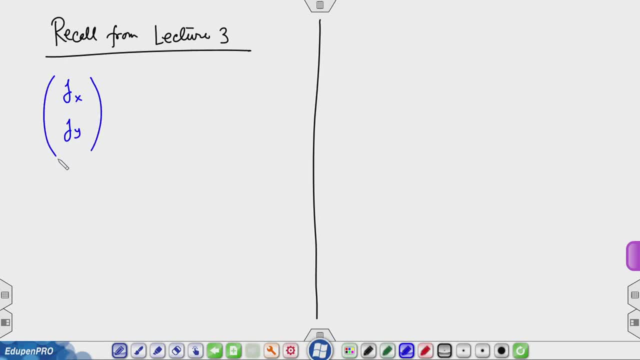 geometry that I have made earlier. J x, J, y is given as sigma naught over 1 plus omega c tau square. 1 minus omega c tau. omega c tau 1 times e x, e square. So that is a very. If I go back to the geometry, what I am considering is this geometry where we have applied a field. 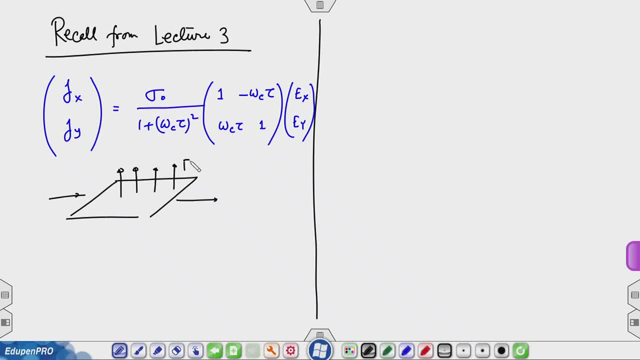 on this two-dimensional gas. and there is this E, x, then there is the. this is the kind of currents you get Here. sigma naught is n, e, square tau over m, And from this one can also calculate the resistivity tensor. 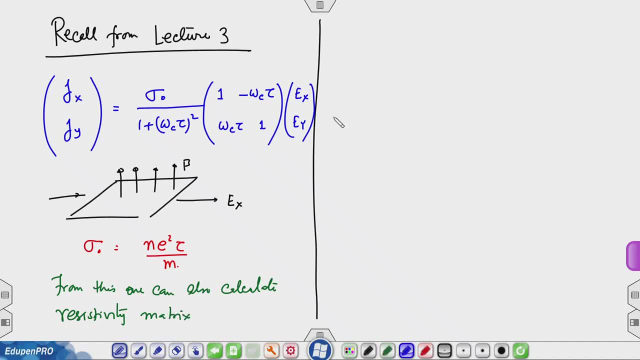 So I am going to call this the conductivity tensor: sigma x x, sigma x y, sigma y x, sigma y y, and inverse of this is going to be resistivity tensor: rho x x, rho x y, rho y x, rho y y. 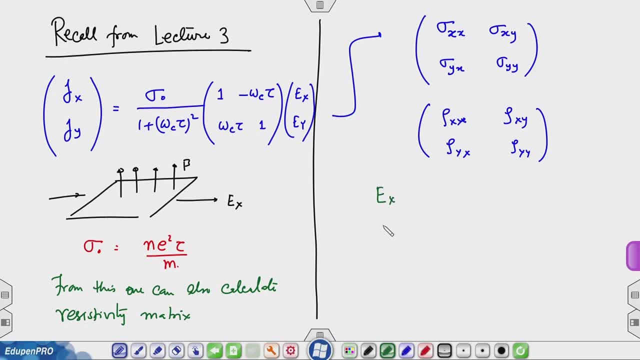 Such that if you take E x, E, y in such a sample, it will come out to be rho x x, rho x y, rho y x, rho y y times j x, j y, Omega c- here is the cyclotron frequency, which is E b by. 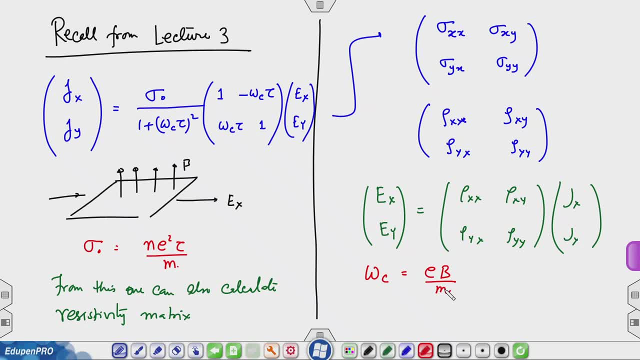 m And omega c is the omega c. here is the cyclotron frequency which is E b by m And omega c. here is the cyclotron frequency which is E b by m. And for traffic signals, for a field of 1 gauss it comes out to be 1.6 times 10, raised to. 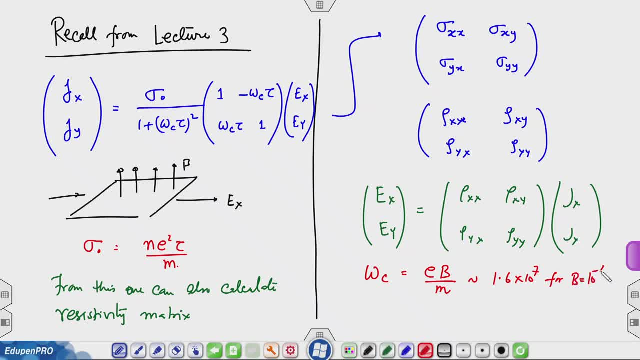 7, for b equals 10, raised to minus 4, Tesla. If you go to very high fields, omega c becomes very large and that is what we want for observing quantum Hall effect. So for example, if you take b equals 1 Tesla, then omega c will be 4 orders of magnitude higher. So thisllen thepod is. 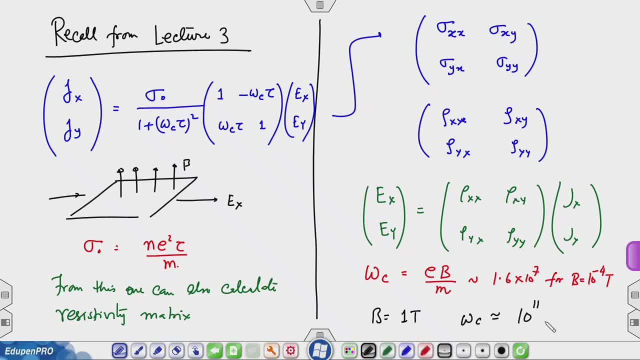 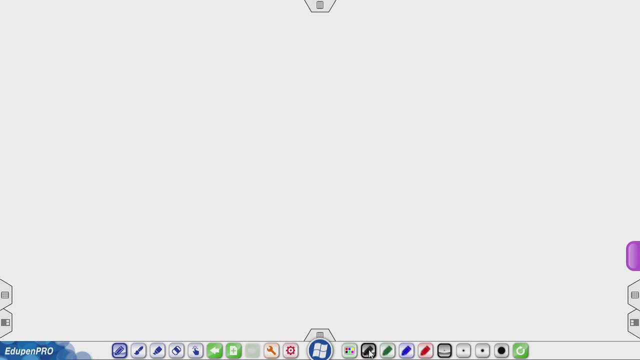 equivalent to R, just like b asked for the formula for the escola And for circuit. if you have 4 orders of magnitude higher, 10 raise to 11 radians per second. So what we have written is that in this whole geometry I have sigma matrix, which is sigma x, x, sigma x, y, sigma. 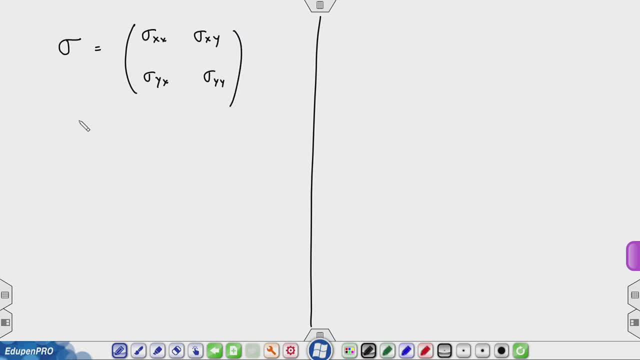 y x, sigma y y, and rho matrix, which is sigma inverse matrix, which is equal to rho x x, rho x y, rho y x, rho y y. So I would like you to do something here. derive rho x x, rho x y, rho y x and rho. 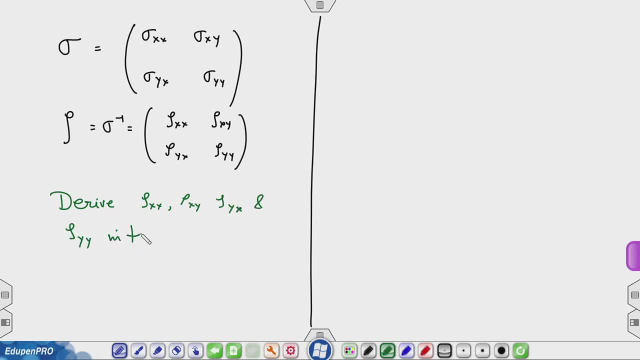 y y in terms of sigma x x, sigma x y, sigma y x and sigma y y And, more importantly, show that sigma x- x equals 0 also implies rho x x is 0.. Similarly, sigma y y- 0 is rho y y 0. 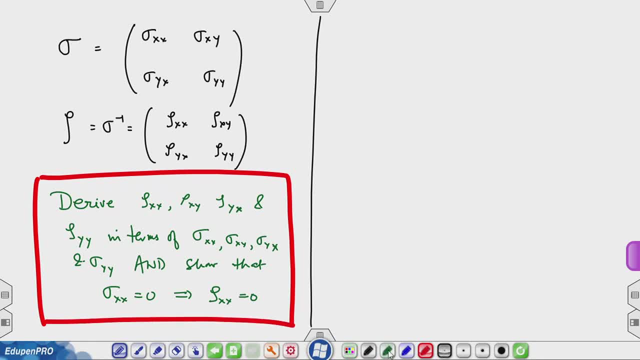 1, 6, 7, 1, 8 and 9, And what that means is that in Hall geometry or Hall experiment, zero conductivity implies zero resistivity. It is very strange, but we will understand that. I want to work in. 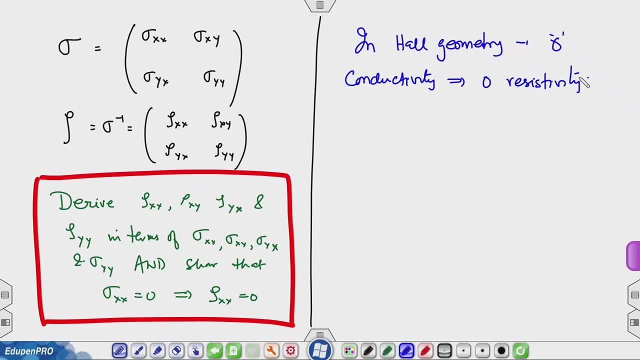 the limit of omega c tau much greater than 1, just to just to make life simple and to give some physical interpretations. but you show it in general. So I am going to work in the limit omega c tau much, much, much greater than 1 and I will show all this. But 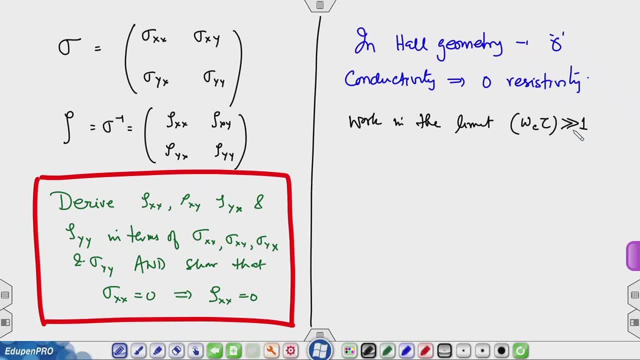 I do want you to work out the general thing. Let us say: sigma naught over 1 plus omega c tau square will become proportional to tau over tau square, which goes to 0, omega c tau square as omega c tau goes to infinity. 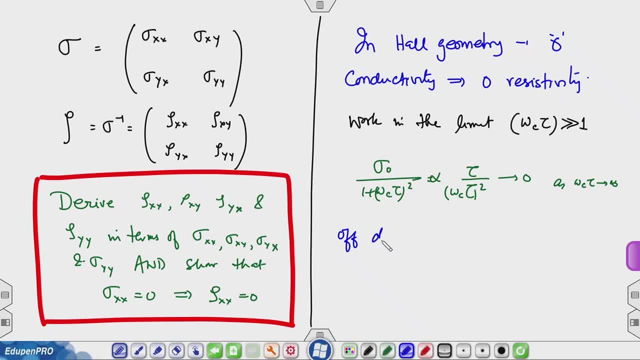 And the off diagonal terms. And now sigma x, y, which is proportional to omega c tau over 1, plus omega c tau whole square times. sigma 0 will go to N, e square over e, b …. 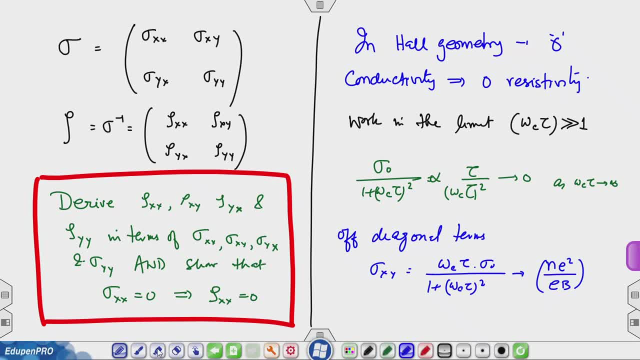 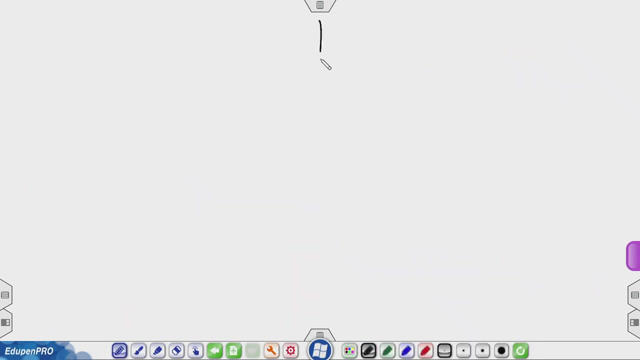 this is no E square, so I will erase this. This goes to N? E over B. So what you can write in this limit, in the limit of omega C, tau, much, much, much greater than 1, what you can write is that J x, J y is equal to first term we showed is 0 minus N? E over B. 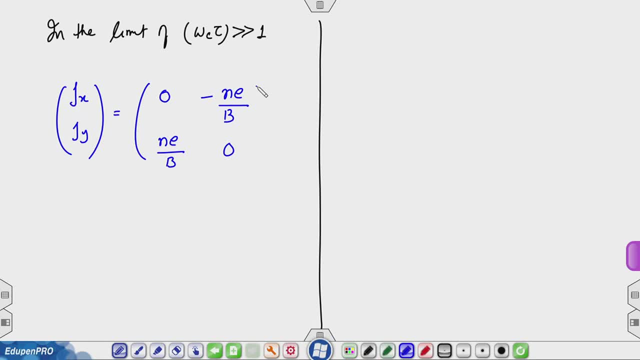 N? E over B, 0, E, x, E, y. So what we have here is that sigma x- x is 0, sigma x- y is minus N? E over B, sigma y x is N? E over B and sigma y- y is 0.. And J x is equal to first term we showed. 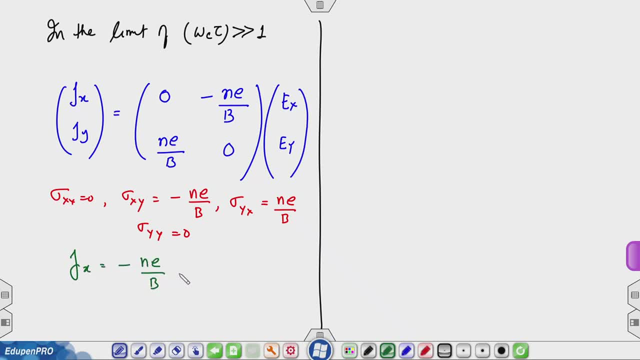 is equal to minus N E over B E, y, J, y, is N E over B E x, the corresponding resistivity tensor. this is- this is just for completeness, you can see it otherwise also- is also is going to be 0, minus B over NE, B over NE 0. This is just inverse of that matrix. 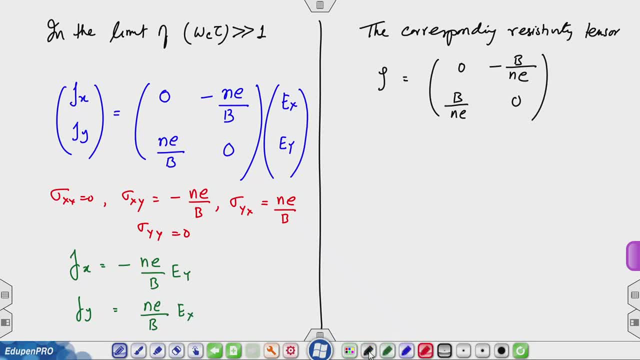 Let us understand this physically. Point number 1, omega C. tau is much, much, much greater than 1 implies tau is tending to infinity for finite omega C, So there is hardly any scattering. And then what is happening is, if I apply a field in the x direction- suppose I have- 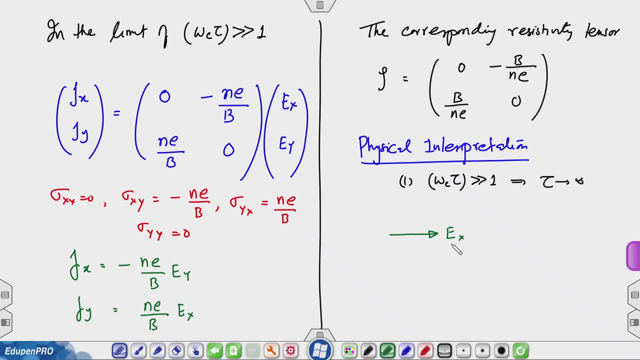 a field in the x direction and there is this B which is coming out, Then an electron would travel in this direction with V equals EX over B and that implies a current движ equals NE V, which is EX over B. Similarly, 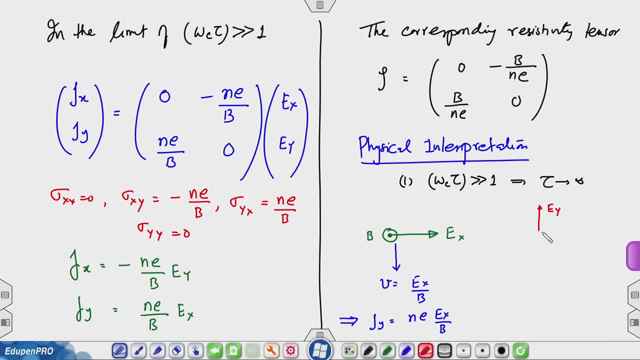 if I have an E, Y and the field coming out, the electron would travel in this direction, will drift in this direction, with V equals 2.. E x over B, Vx, E, y over B, which will give you a current in the negative direction. J, y equals minus. 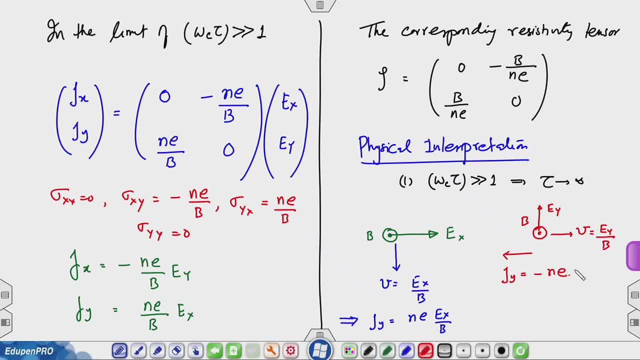 N, E, E, y over B. that is what it is. So, if there is no scattering and you have this geometry, where you have this plane perpendicular to which you apply a magnetic field, which is the Hall system, and you apply these fields, the current, in the x direction, in which you 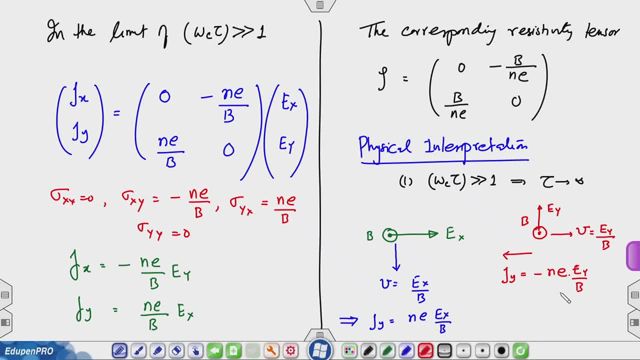 are applying, the field is 0 and current in the perpendicular direction is non-zero, and that immediately tells you why the conductivity in the direction of the applied field, applied E- X is 0, sigma x- x is 0 because current in that direction is 0.. Whereas sigma x- y is. 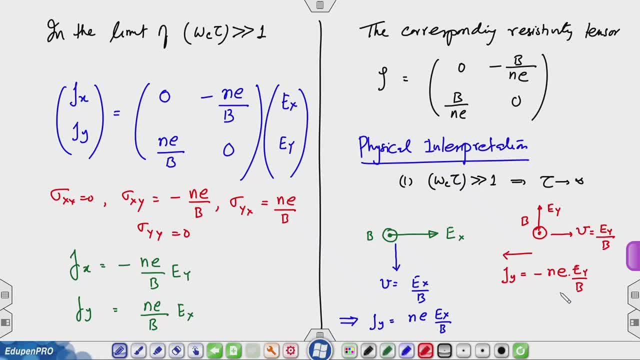 non-zero, because when you apply the field E- x, you get a current in y direction. Similarly, you can see that if there is a current in the x direction, the field is 0 in that direction and therefore rho x- x is 0.. 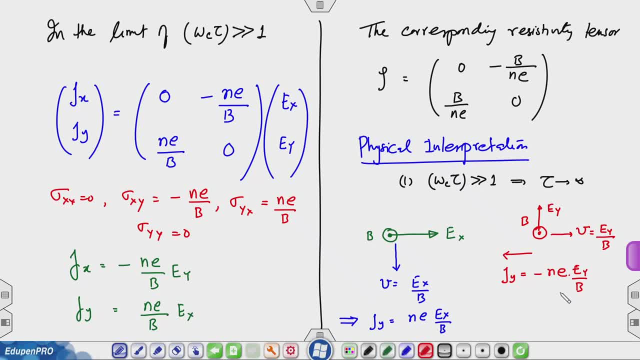 So I will let you think a little more About it. I have explained physically what it means to have the rho x x and sigma x x, both 0, 0 conductivity implying 0 resistivity, and vice versa. So let me now leave you with 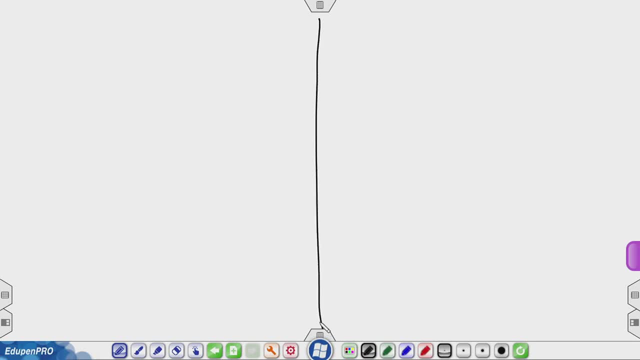 this thought about this Interpret how. 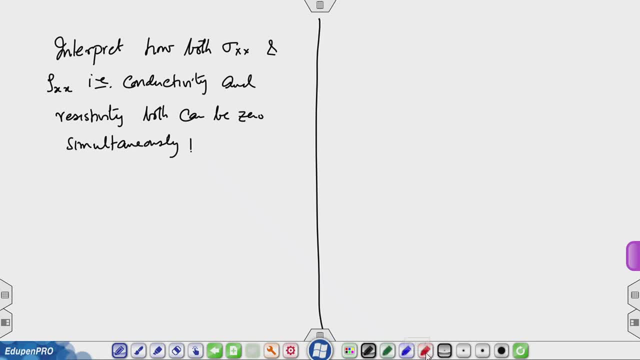 We have discussed this, but I want you to think a little more about it. So that is one very strange thing about whole experiment. What comes out is that if I look at one of the j say j, x, this is equal to n, e over b, e, y- forget about the sign right now, or? 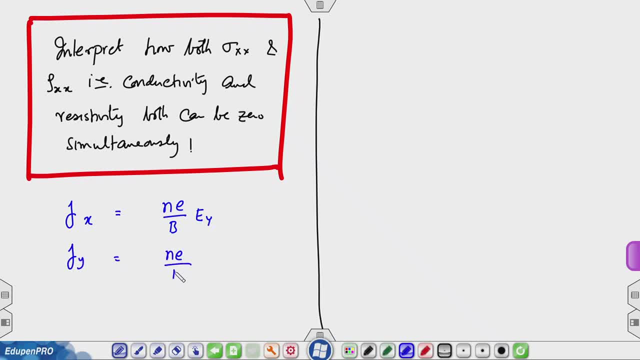 j y is equal to n e over b e x and the resistivity is opposite of that. So I have e y equals, That is, b over n e j x, and e x equals b over n e j y. So resistivity rho x, y is equal. 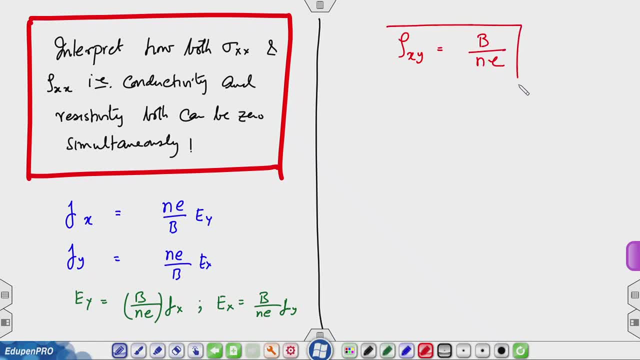 to b over n, e. That is the whole resistivity. Now let us see what happens quantum mechanically or in the experiment. So experimentally one observes that rho x, y is equal to h over e, square, 1 over nu, where nu is an integer. So if you want to understand quantum Hall effect you have to 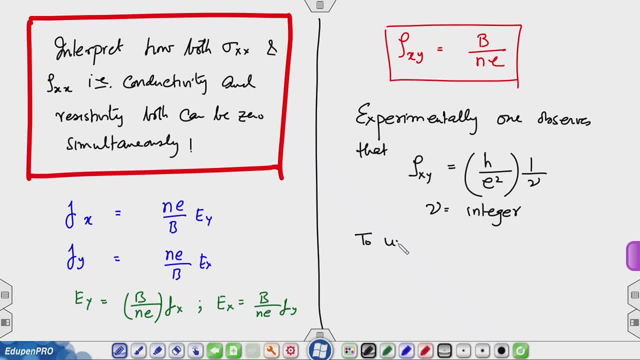 prove that. So to understand quantum Hall effect, or integer quantum Hall effect, we must have n equals e, b over h times nu. If you have that and put it in the restaurant in this formula this leads to this formula. So our job is now going to be that in this, 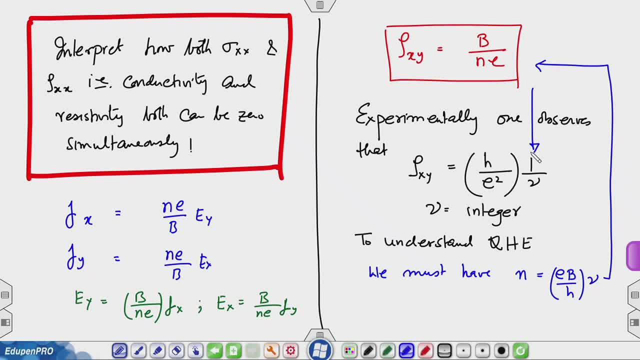 two-dimensional system. I show that the electron density, or the electron density per unit area, because we are doing experiments in two dimensions- is going to be proportional to B, proportionality constant being E over H. and then you multiply it by an integer. If we can show that, our 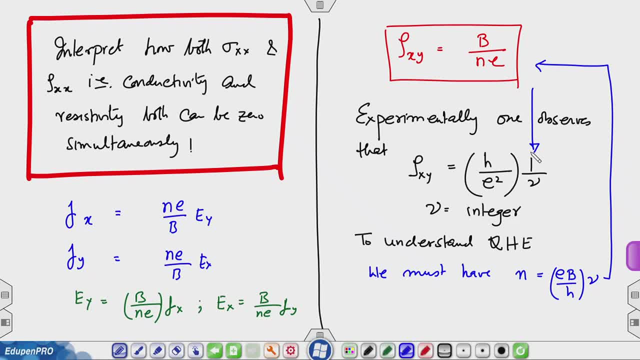 job is done. That shows you that rho xy is going to behave H over E, square times 1 over the integer. The other thing you have to explain is that when that happens, that time the conductivity is going to be 0, there is going to be no current in the direction of applied field. 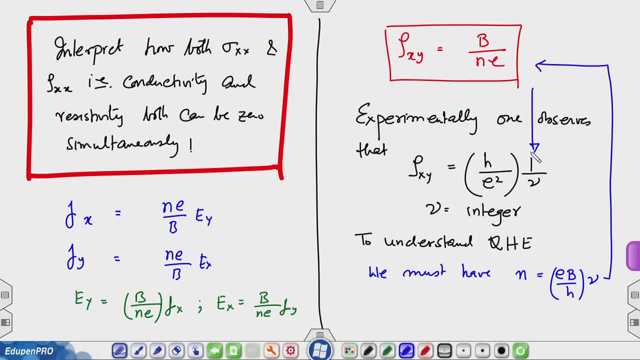 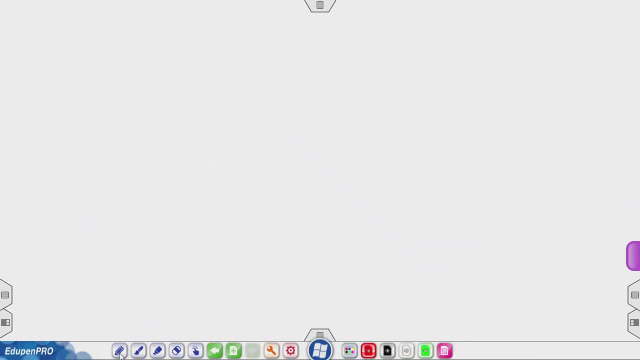 So this is going to be our job. With this background, I want to explain this and I will provide a few concepts. So that is what I am going to do in this lecture and next lecture. we will then bring it all together to get integer quantum Hall Effect. 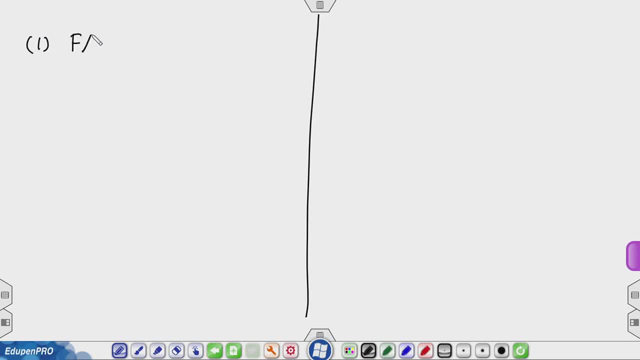 One concept that I will need is that of flux: quanta, FLUX, QUANTA, FLUX QUANTA. What you can show is that flux through a ring carrying a current comes in quanta of H over E. So if I have a ring and I apply magnetic field, the flux through this ring will be 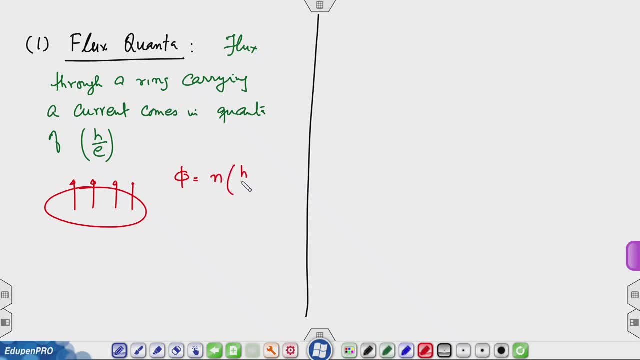 equal to N times H over E. So this H over E we are going to call phi naught, or this is quantum of flux. This comes about because you want wave function. psi should be such that psi at phi is equal to psi at phi plus 2 pi or 2 N pi. So this uniqueness of the wave function gives you 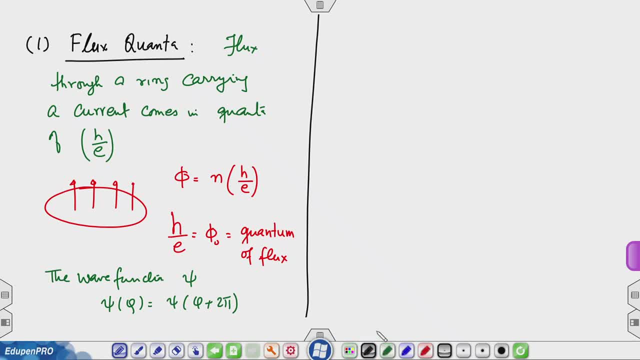 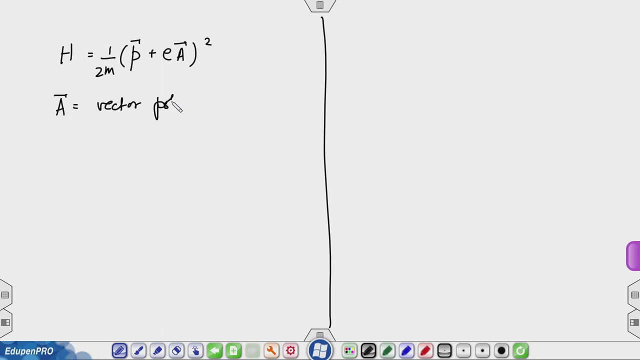 flux, quantum. So learn about quantum of flux. You must have done it in your quantum mechanics course. And second thing that I am going to spend considerable time on is a motion of quantum. 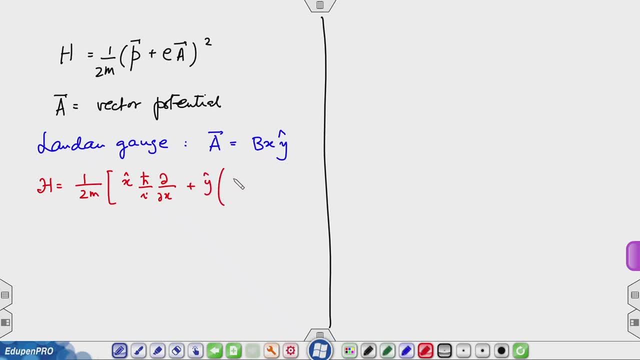 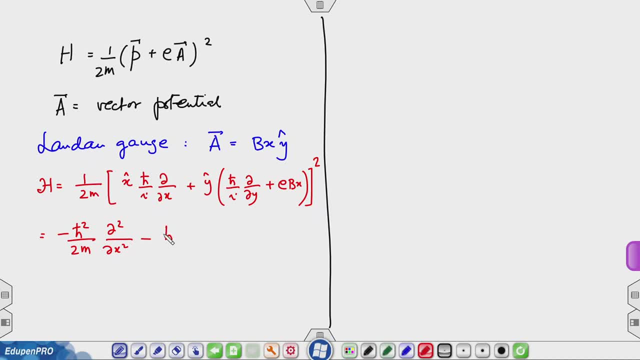 This is the equation that I am solving By looking at this structure and, since this has been solved many, many times, I can immediately make an answer for the wave function psi x. 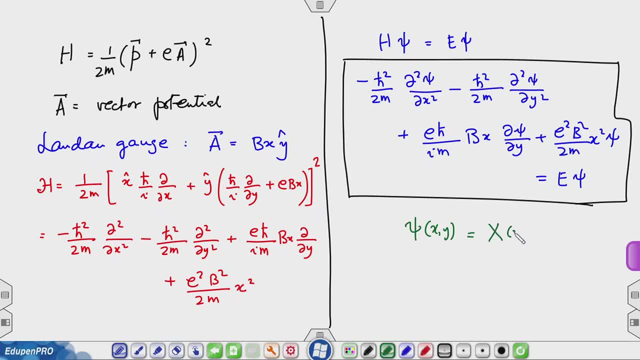 y is equal to some x part times e raise to i, k, y. This happens to be an Eigen function. This is by looking at the structure and since I want to normalize the e, k, y part, I will also multiply it by 2 over l y. I think it is 2 root, 1 over l y. Since this is normalized. 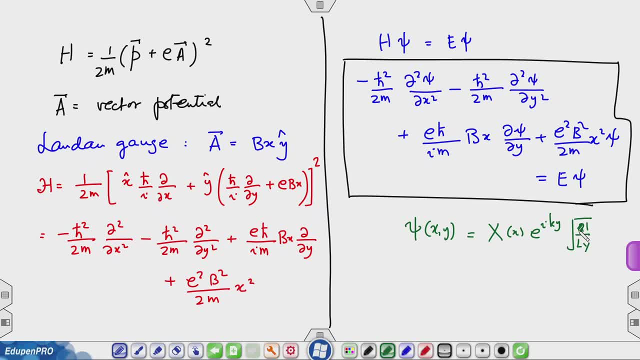 over the length l y. Now, if I substitute this n, then I mean I can. I can act on e, raise to i k, y when d by d y gives you i k double derivative with respect to y, gives you k square, And therefore, 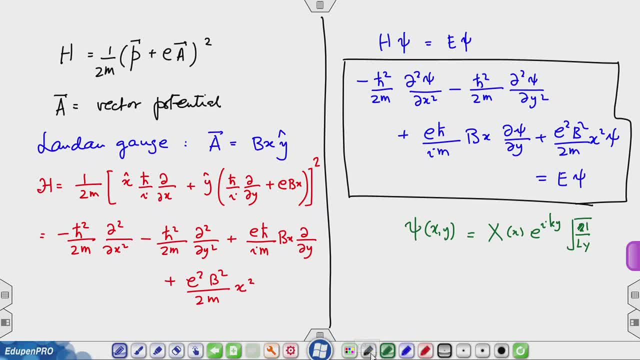 what you get is when you substitute minus h cross square over 2 m, d 2 x over d x square Plus h cross square k, square over 2 m, that is from the second term, plus e h cross k over m, and this is all multiplied by x, multiplied by x, and there is a, b, x also here There will 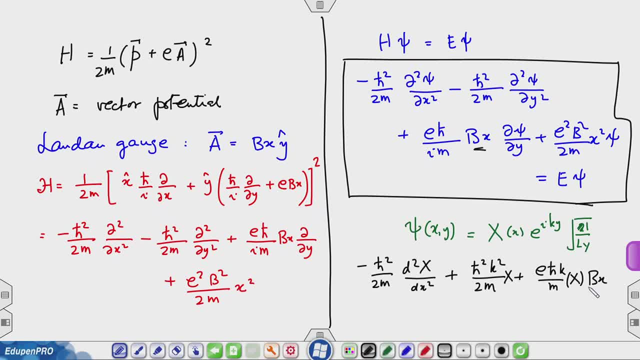 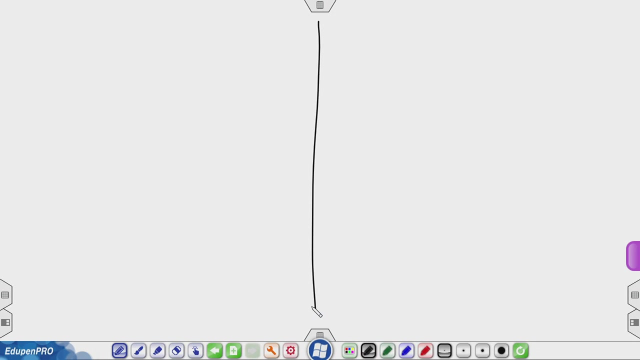 be a b x Plus e. square b square over 2 m x. square x equals e x. That is the equation you get for x. So let me write it again on the next slide. So equation for x that I am writing. 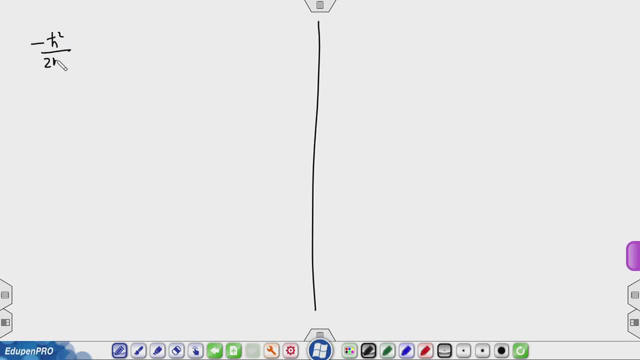 is minus h cross square over 2 m d 2 x over d x square. plus h cross k over 2 m d 2 x over d x square. So h cross h cross square. plus h cross square k square over 2 m x plus e h cross k over. 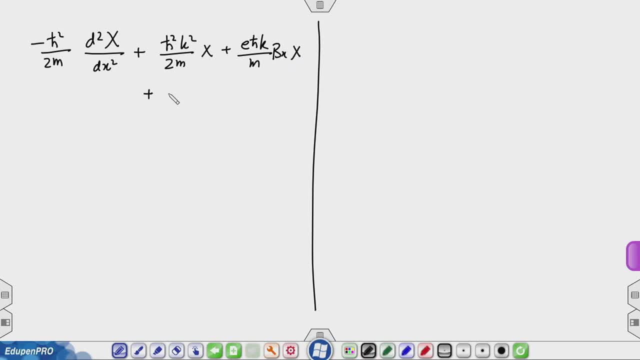 m, b x x plus e. square b square over 2 m x. square x equals e x. Complete this square and you can write this as: minus h. cross square over 2 m d t. square x over d x square. that is sin d- x And some Faster casue. why don't I just write that here? This is a rather complicated. 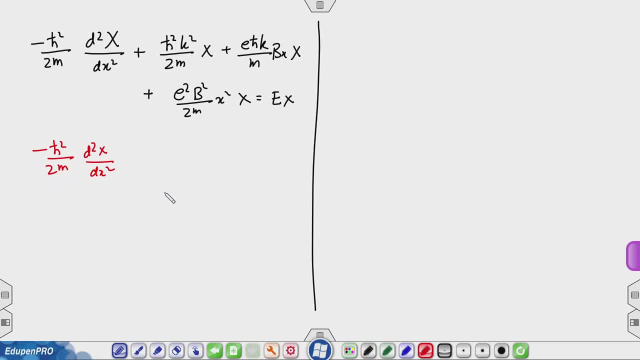 d 2 x over d x square. In the second part I take out 1 over 2 m and then complete the square. I get h cross k plus E b x square. x equals E x. I can take E b out and write this: 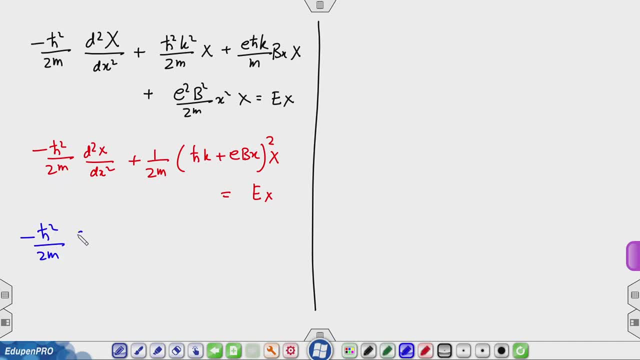 as minus h cross square over 2 m. d. 2 x by d x square plus E square b square over 2 m. x. plus h cross k over E b. whole square equals E x. This is the equation For a simple harmonic oscillator, with the second term on the left hand side giving you. 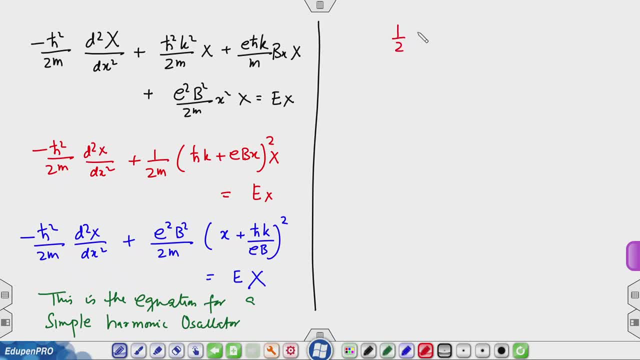 the half k x square. So half k x square, which is also one half m omega square. x square, like 1, is actually replaced by one half m E b over m square and inside I have k plus h cross k over E b whole square. So this is omega square and this is shifted harmonic oscillator. 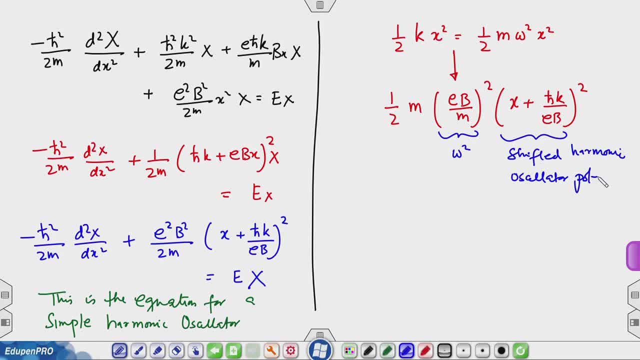 But now what happened When I took the equation? the first time I took the equation, I really want to use the first one to find it out, the extrapolation of the equation. so let me, unfortunately, also introduce to you the вариант of the equation. 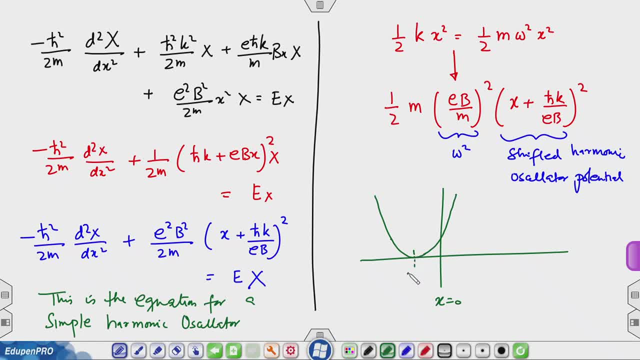 So before we do the warded randomization, let us see the fiance of the equation, Such A A minus A, 1 A. That was the case, right, and this is one half m omega cyclotron, square x square. this is the cyclotron frequency. 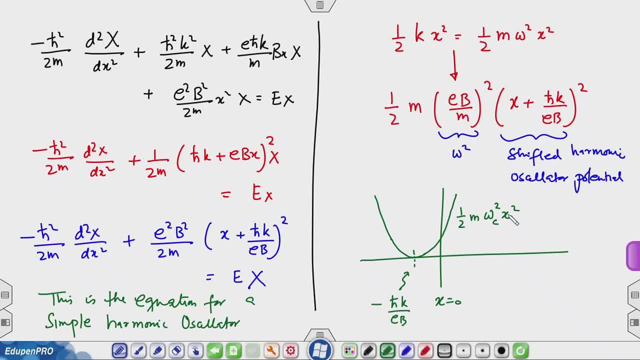 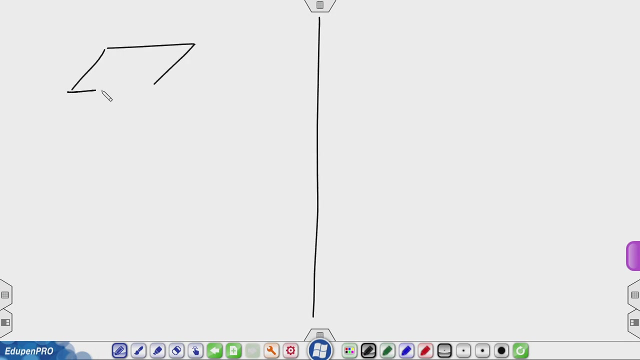 Solution for this is very clear. So the solution is going to be the psi harmonic oscillator and Eigen values E, n are going to be n plus a half, h cross, omega c. Let me repeat myself on the next slide. So when we had this system of 2 D gas, in which 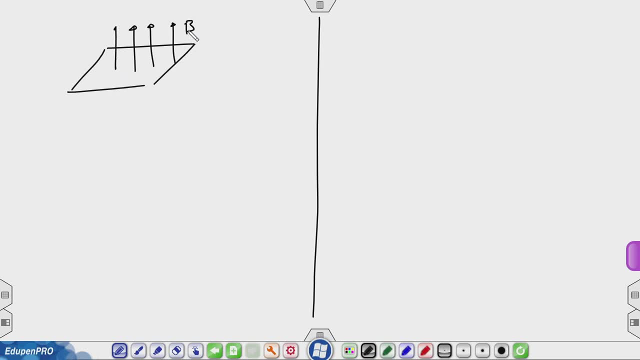 we have applied a magnetic field B in the z direction and I am working in Landau gauge where I take a to b equal to b, x, y, I get the equation where h x equals E x or h psi equals E psi, where psi is x, e raise to i, k, y root 1 over l y. 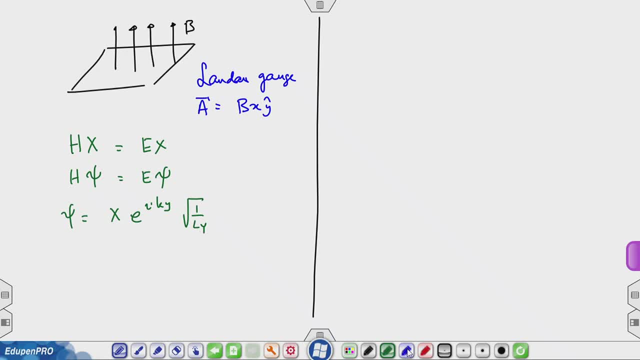 and x satisfies harmonic oscillator Schrodinger equation with the potential of the particle being. let me make that this is: x equals 0, the potential is shifted potential. So this is dis dando a potential. this is minus h, cross k over E, b and this potential is one half m omega c. 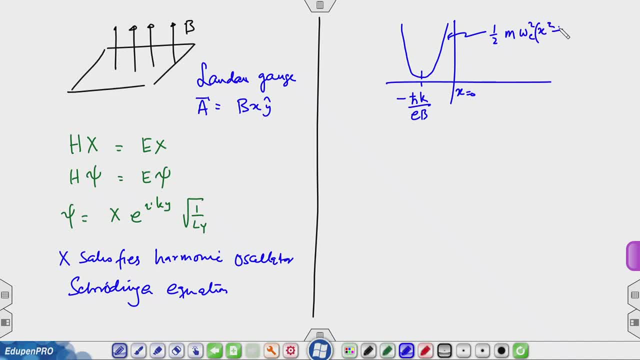 square. x plus E- h cross over- sorry, plus h cross k over E b whole square. This x is food. x square will not be there. So the wave function x is psi x- n- harmonic oscillator and the total wave function psi x- y, which is a wave function of n and k, is equal to psi n- x- harmonic oscillator. 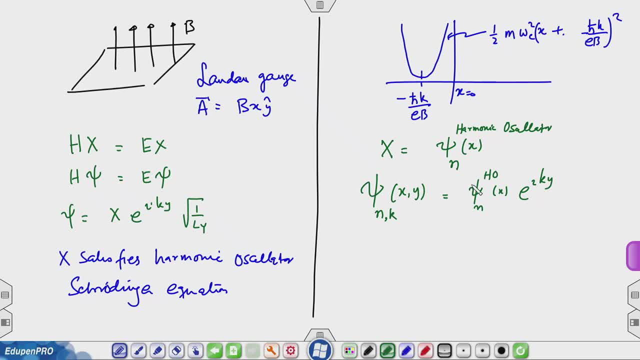 times e raise to i, k, y and there is this normalization constant square root of 1 over l y. We are taking periodic boundary conditions over k, So psi n k is equal to n plus a. half h cross omega c. This is very important to understand. 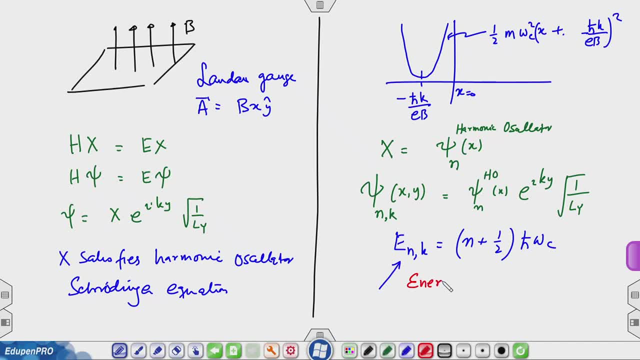 that energy is independent of k. Since energy is independent, that means it is a highly degenerate level, because all the k values that are allowed are going to be in this level. So all that k degeneracy, energy is independent of k, but you do have k coming. 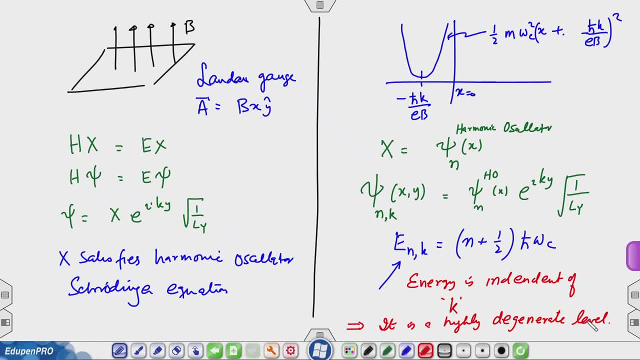 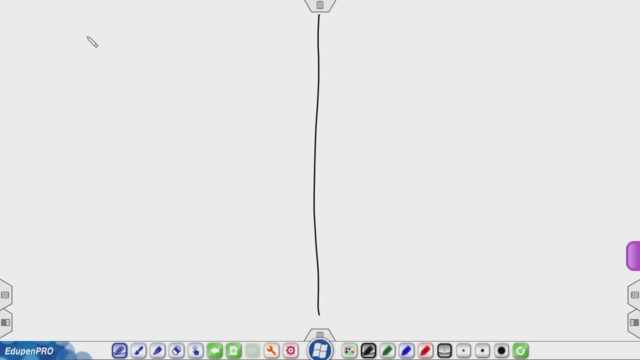 in the wave function. So all those k's are going to come into this, and that is the degeneracy. Let us see how that comes about. So what we have is- that is why I kept making this picture of the harmonic oscillator- is that the x naught by which this, this potential? 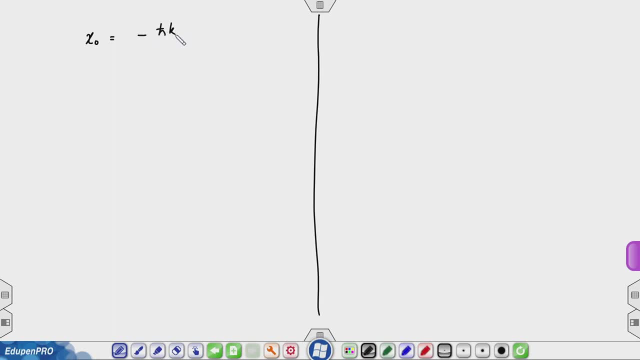 shift is minus h, cross k over e, b. So your potential in this strip of metal is forward, about here, centered about here, depending on different k's. So you may have a potential like this, you may have a potential like this, you may have a potential like this and like: 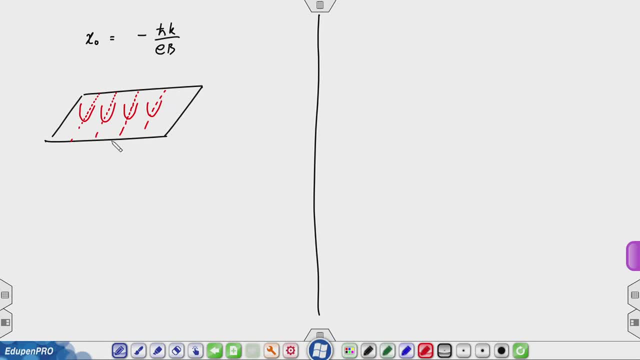 this for each k value. this is for each k value, And all these have the same energy: E n. So whatever the number of k values are, that is going to be the degeneracy. I want you to first tell me this difference. 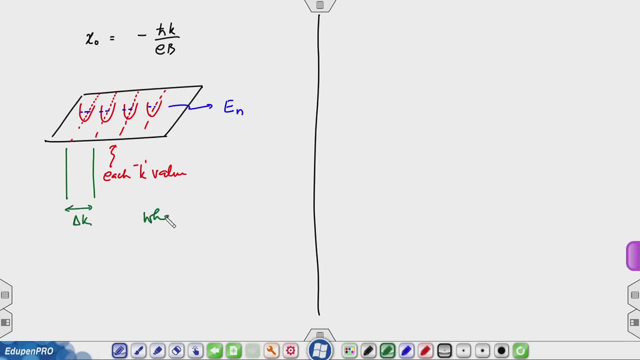 Suppose this is delta k. what is the value of delta k? So you have these wave functions which are like this: I have psi n, So delta k, x, y equals psi. harmonic oscillator n, x, e raise to i, k, y square root of 1 over. 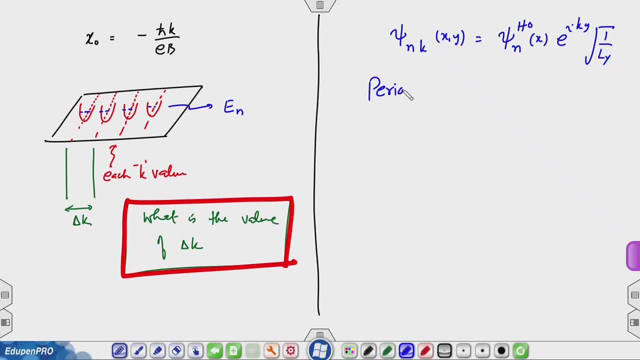 l y and periodic boundary conditions over l y. give me: k equals 2 pi over l y And this is going to be an n. So you have different k values. Now if the sample size is l x. if the sample size is l x, then k maximum magnitude is equal to 1 over l y. So 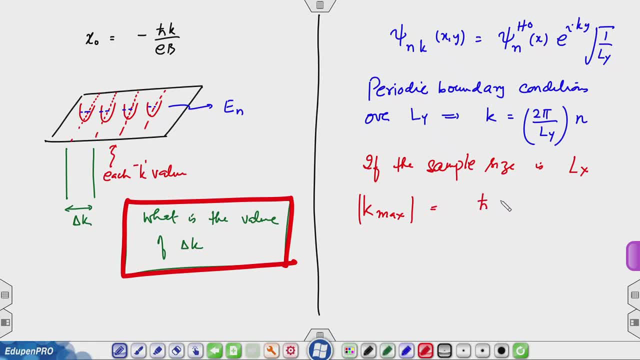 remember thatар y is going to be equal to k l t. all right. So l x is going to be equal to h cross psi. k max over e b equals l x. that is why is going to satisfy, So k max satisfies. 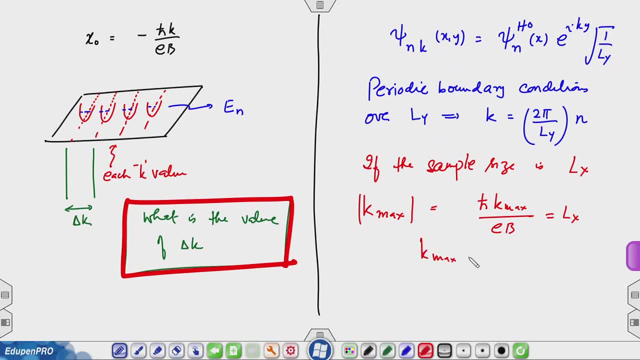 this. So k max is going to be e, b, l, x over h cross And The number of levels up to k max are going to be E, B, L, x over h cross, times, L y over 2 pi. That is the density. 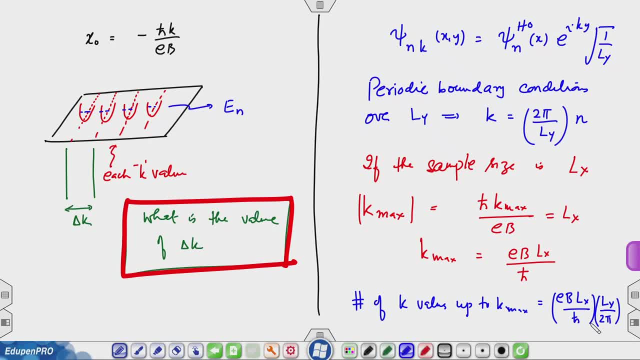 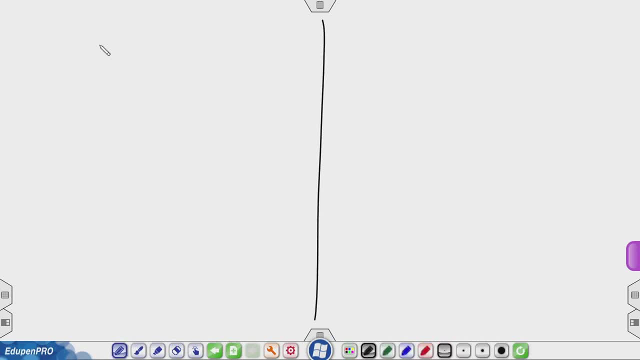 of k points and let me repeat this point. So you have this strip with length, L x, width, not width but L y, over which I have the periodic boundary conditions. The wave function psi x, y depends on n and k Is equal to psi n. harmonic oscillator x times E raise to I k y root 1 over L y. The k values. 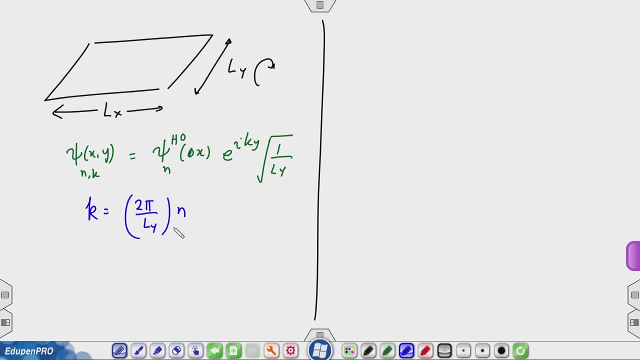 are going to be 2 pi over L, y, n and k max is such that E k max is on the negative side. but that is ok. So h cross, k max over E B is equal to L x. So k max is equal to E B, L x over h cross. 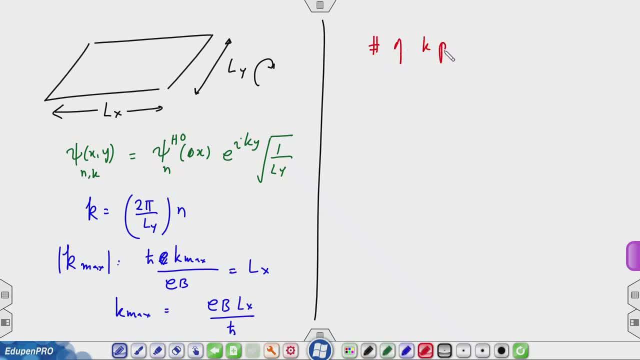 and so number of k points is going to be equal to density of steps in k, See density of steps in k times k max. And density of steps is L? y over 2 pi times E, B, L, x over h cross, which is E, B over h, L, x, L, y, L x times L, y is the area. So this is: 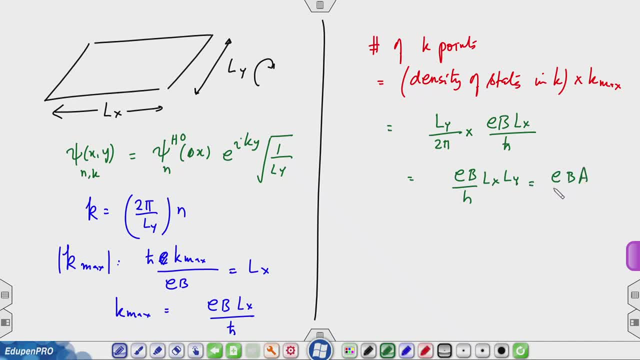 equal to E B times the area over h. Now recall quantum of flux phi naught is equal to h over e and here flux through the level is B, A. So the degeneracy of each Landau level is phi over phi naught or it is equal. 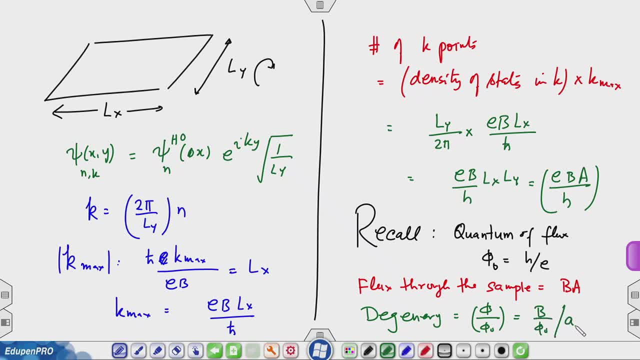 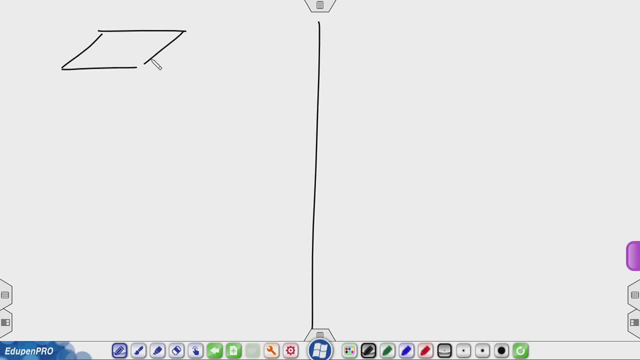 to B over phi naught per unit area. That is the degeneracy of Landau levels. So what we have obtained is that when I put a sample in a magnetic field B, you have these oscillator wave functions. 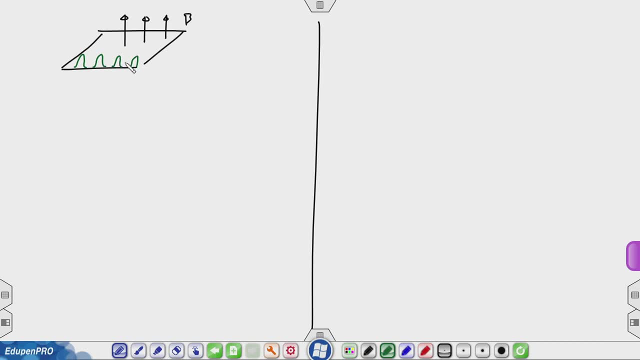 separated by delta k, which I have asked you to find out. and all of this have degeneracy. we have. here was a describing this. 翻 N will be characterized for the energy levels of this. So in the sampling you have these energy levels. n equals. 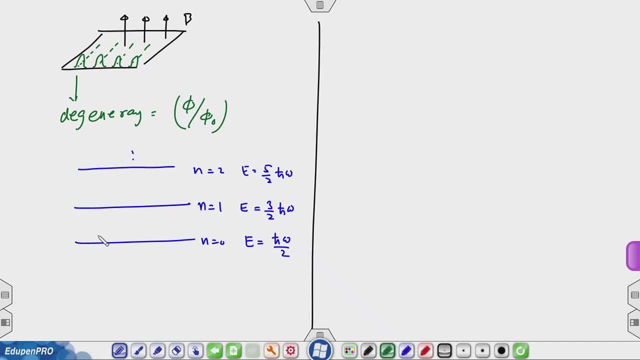 omega and so on, and each one of this has these tons of levels. So all those k levels have come into this and notice that k is negative. So you have in the sample electrons having this velocity V equals h, cross k over m and in the x direction, this wave function. I am. 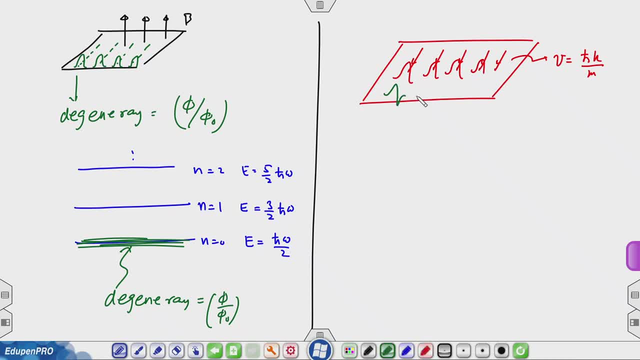 showing only the ground state. you could also have the first excited state, the second excited state and all of them are degenerate up to this level: phi over, phi naught. So that is one thing that I have talked about. Now let us ask the question: what happens if there is a field E applied in x direction? 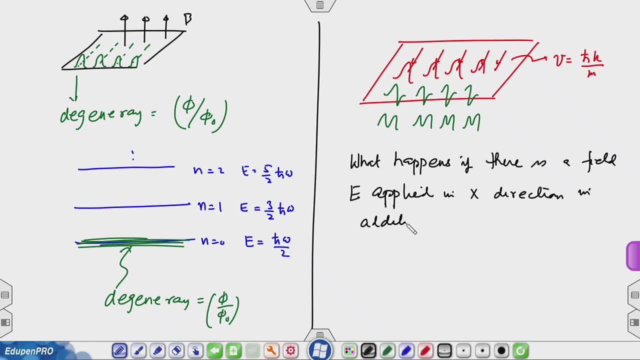 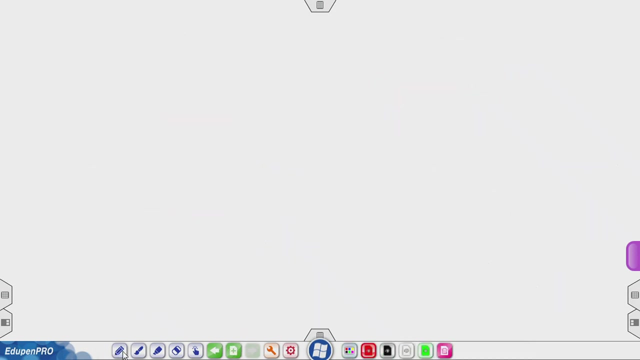 in addition to B, Perpendicular to the sample. So what you have is: here is the sample, here is B, and you have also applied an Ex. So the Hamiltonian now is going to be equal to P plus E. a square over 2 m charge is minus. 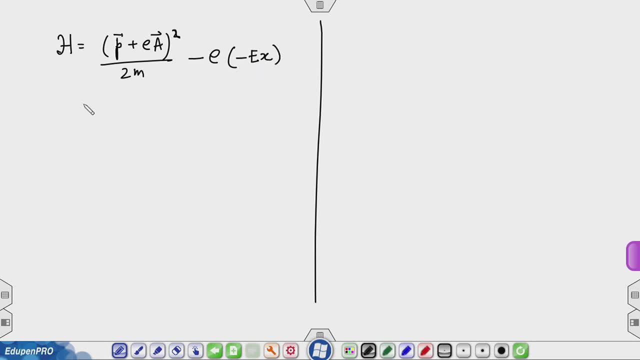 E potential is minus E x. So this is going to be P over E, a square over 2 m, plus E e x. So there is this additional term to the previous Hamiltonian. Work it out that I will leave for you, because you are just adding this term. 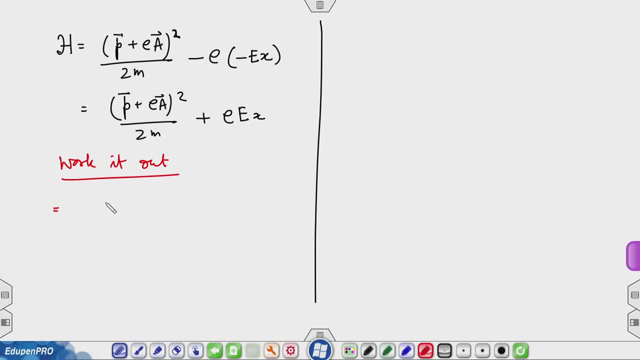 And what you are going to get. this Hamiltonian, as is minus h cross square over 2 m d 2 by d x square acting on x plus 1 over 2 m h cross k plus m e over 2 m d 2 by d x square acting on x plus 1 over 2 m h cross k plus m e over 2 m h cross k. 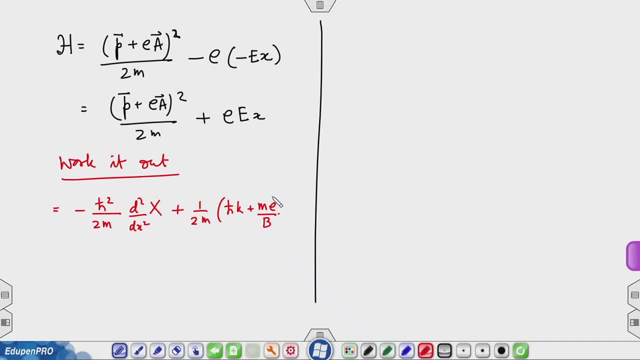 That is the momentum, So let me make it look better: m e over b plus E. b x square. acting on x minus 1 half m e over 2 m. h. cross k plus m e over 2 m. h. cross k, E square over B. square M is on top minus h. cross K. E over B. acting on X. acting on X equals. 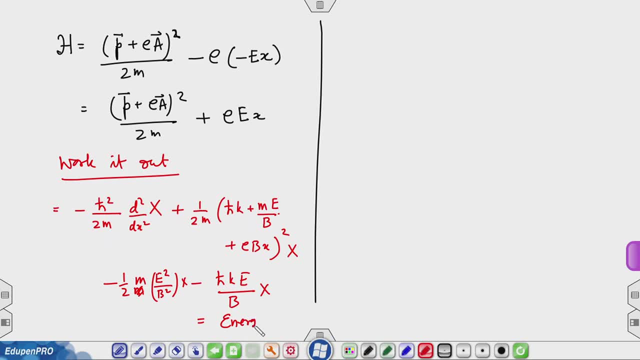 the energy, Since I have used E for the electric field times X, where we have again taken wave function psi X, Y to be of the form psi X, X, E raised to the power of X. So you have to work it out, Put it in the Hamiltonian and see all this. Then I can. 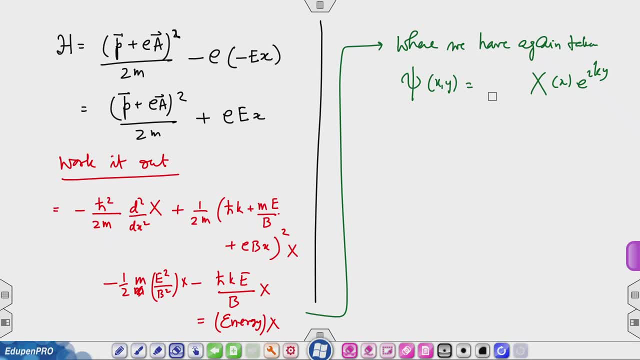 also write this as: by adding half M E square by E square twice. I can write this as: minus h cross square over 2 M. d, 2 x by d x square plus E, square B square over 2 M x. plus h cross K. plus M E over B, 1 over E B, whole square. 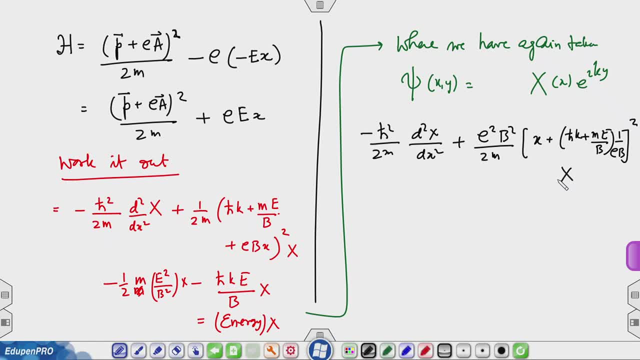 times X minus 1 half M E over B, M, E over B. square X minus h. cross K E over B. x equals energy times X. I will leave the rest of the work out for you, and what you get from this is energy comes out to be N. 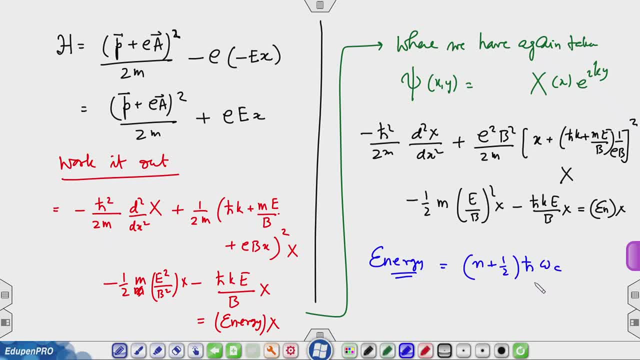 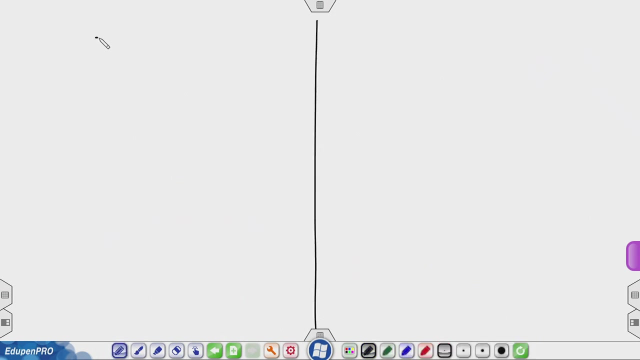 plus a half h cross omega C. Minus E over B h cross K. plus M E over B. plus 1 half M E over B square. You have to fill in the details, So let me write this again: We have this system in which the energy is. 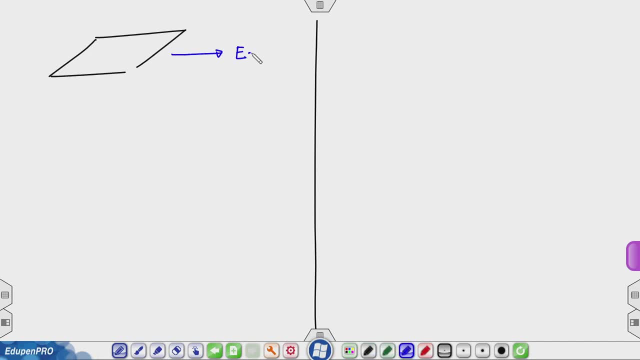 which gives me daran from the bags in the justify we have have to fill in thesedate line du du se plus one half m e by b square. I will give you some work here. interpret each term in. 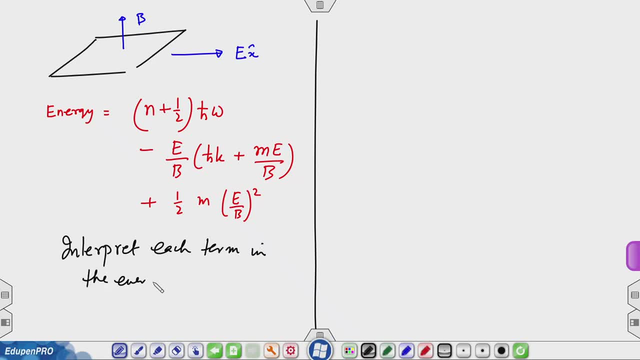 the energy. So you will have to work out things and then see what it means. What is very important here and the that is the important point- that the velocity of the electron Now, which is 1 over h, cross d e by d k- if I think of this as a wave packet now- is in. 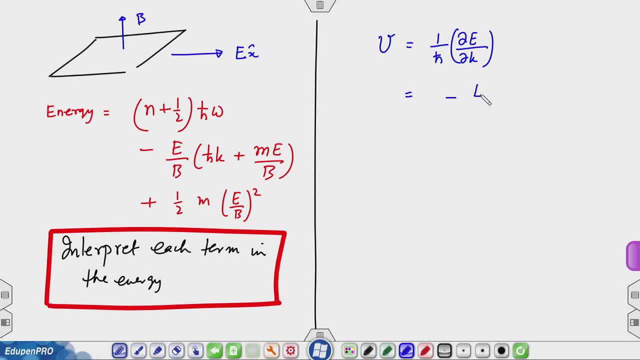 y direction and it comes out to be minus e over b, Since k is the y direction, k, so this is in y direction. So even if you work it out quantum mechanically, what you are getting is that in this system, where you have e and b, perpendicular e is in x direction and there is b, you have electrons. 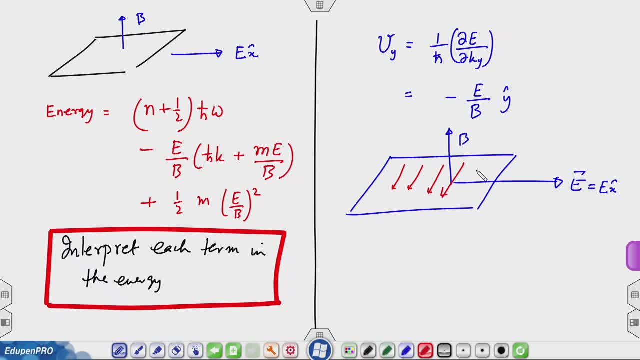 which are flowing this way with velocity e by b, the same as the butcher'swork Because as the classical result. So I have set up a lot of things today for you and I will stop here today by concluding the lecture and then work with these things to explain quantum. 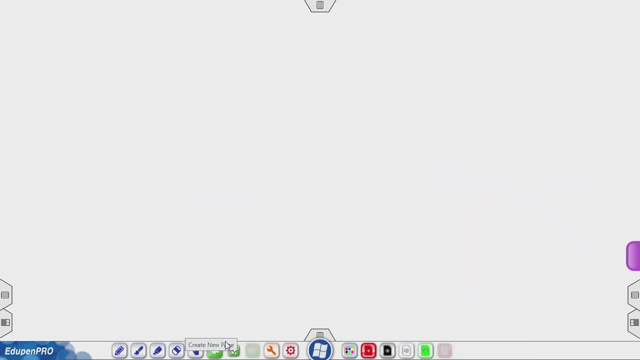 Hall integer, quantum Hall effect in the next one. So let me now conclude lecture by saying that in Hall effect rho x- x is equal to 0. implies sigma x- x equals 0, implies rho x- x is also 0, this you have to interpret.